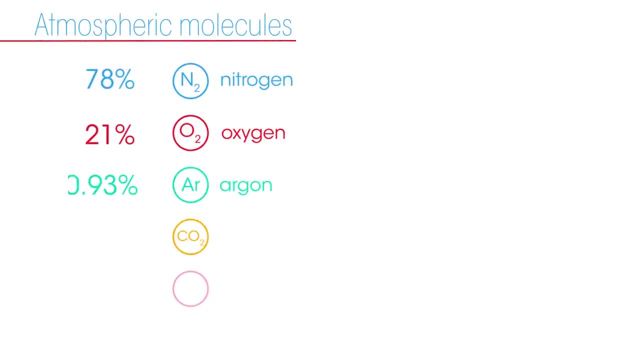 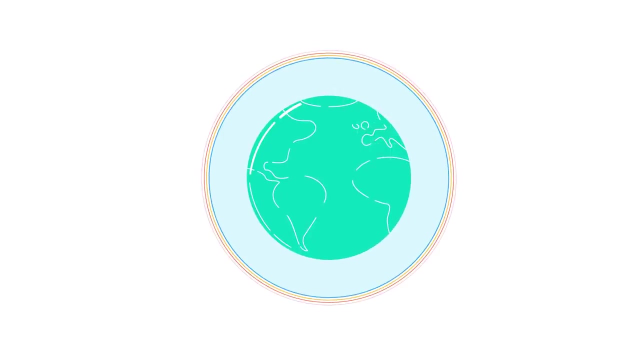 including mostly nitrogen, the oxygen that we breathe, argon, and then carbon dioxide and other molecules in tiny concentrations, including water vapor. As well as providing us with the air we breathe, the atmosphere also protects us from the radiation and the heat of our sun By day. the 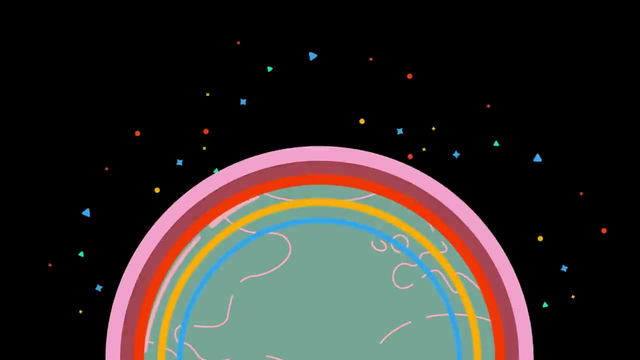 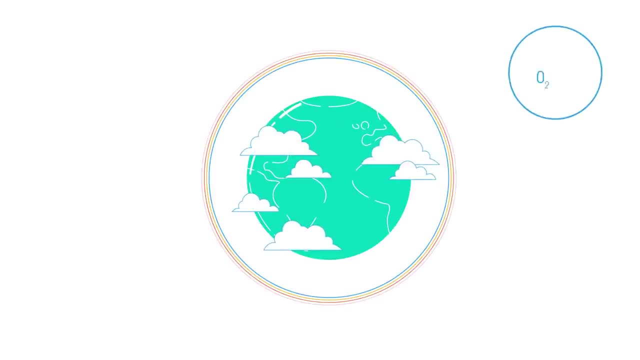 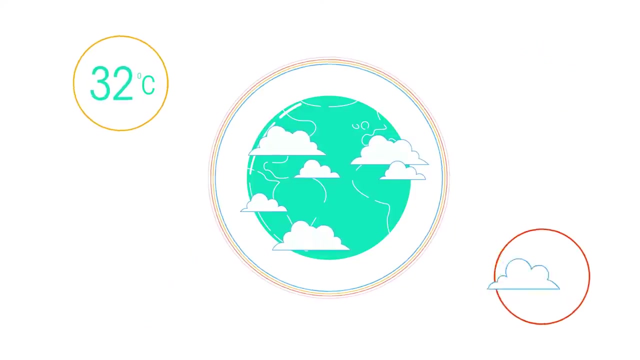 atmosphere stops us getting too hot, and by night it wraps us up in a blanket to stop us getting too cold. It also provides us with all our weather: oxygen to breathe, water, vapor, weather and temperature control. I hope you're starting to see how wonderfully important this blanket of 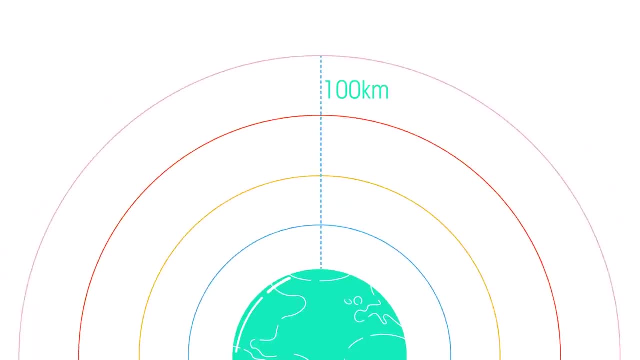 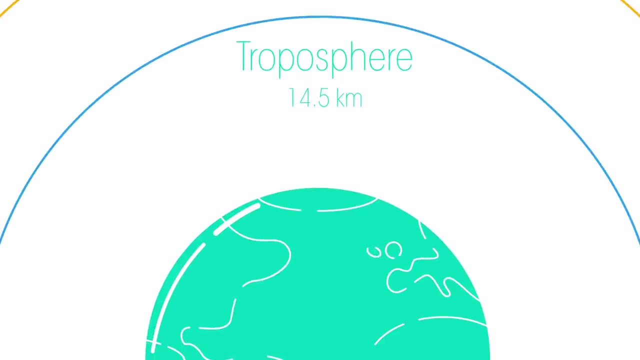 gas is to us. The atmosphere is about a hundred kilometers thick and is broken down into different layers. It starts with the troposphere closest to the earth, which extends to fourteen point five kilometers Thanks to gravity. this is the most dense part and is where the clouds. 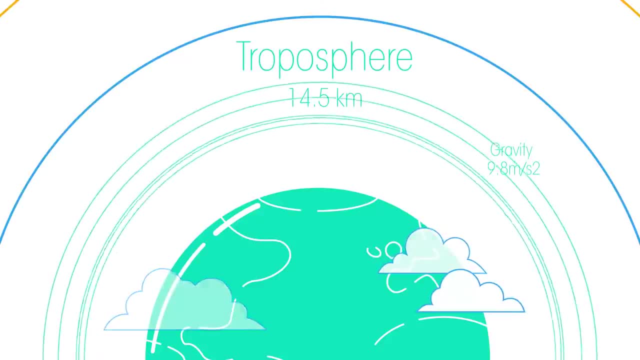 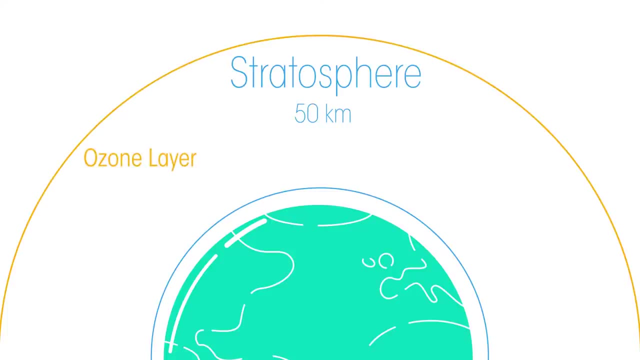 are found. Nearly all of our weather happens in here. Then the stratosphere up to fifty kilometers, which contains the very important ozone layer. The ozone layer both heat the stratosphere and also absorbs and scatters harmful ultraviolet radiation from the Sun. 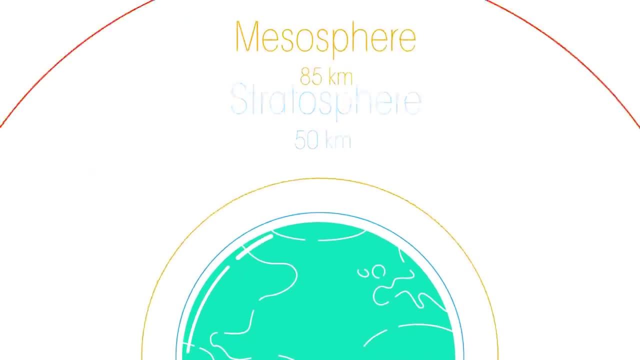 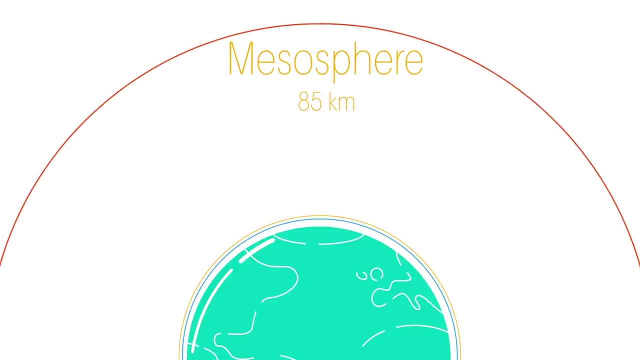 protecting all life on Earth, And beyond that we have the mesosphere up to eighty-five kilometers. The mesosphere protects us from flying pieces of space rock called meteors. When they hit the mesosphere, the friction of the air causes most of them to burn up or, at the very least, to break down. 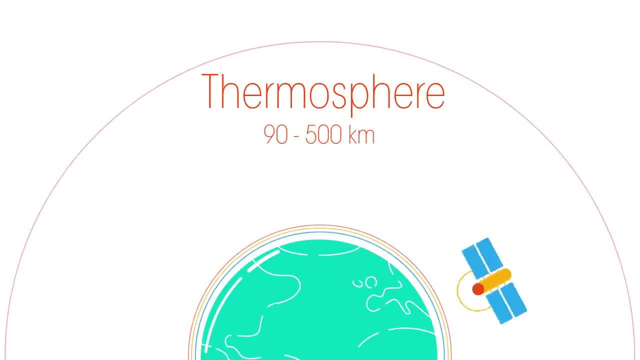 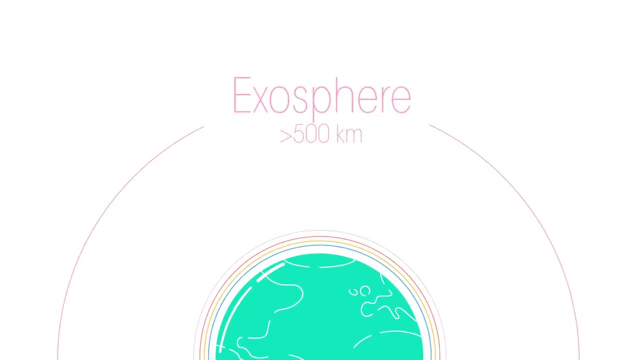 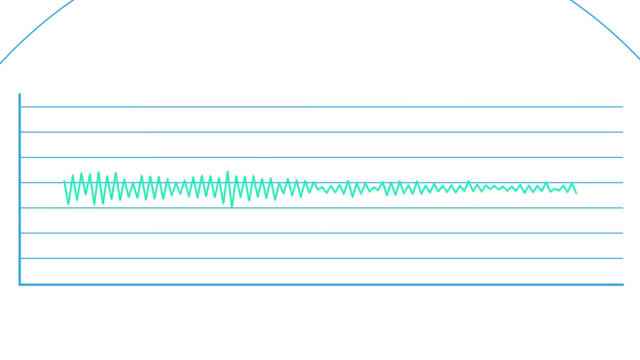 into much, much smaller pieces. Then there's the thermosphere- The International Space Station orbits the earth at four hundred kilometers, and then the exosphere is where our atmosphere merges into outer space. Another wonderful thing the atmosphere does is that it enables us to hear. 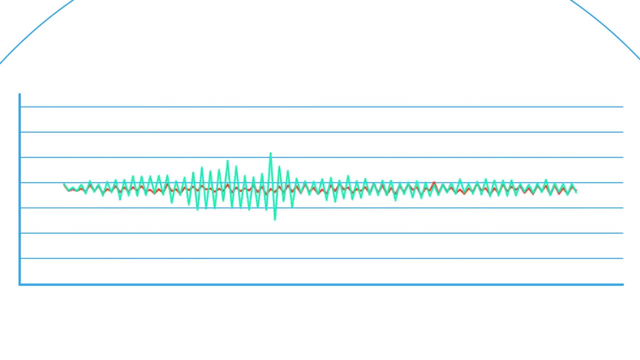 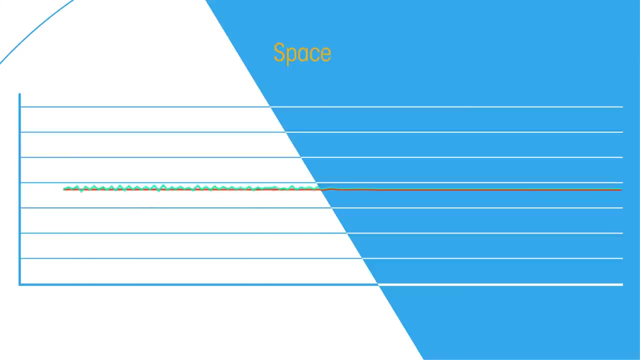 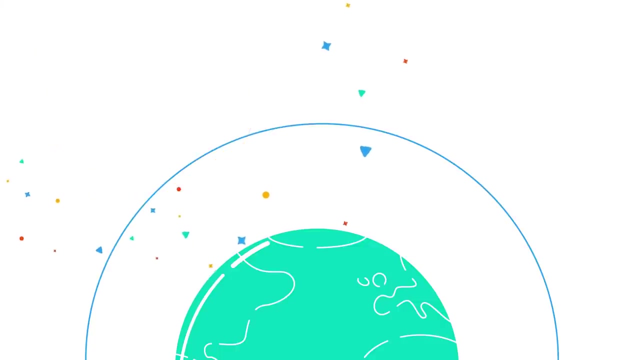 each other, to hear bird songs, to hear cars as we cross the road. Sound waves need air to travel. as there is no air in space, Sound can't travel, so space is silent. Any movies where spaceships leave our atmosphere and explode, that noise is all there is. The atmosphere is a space station. 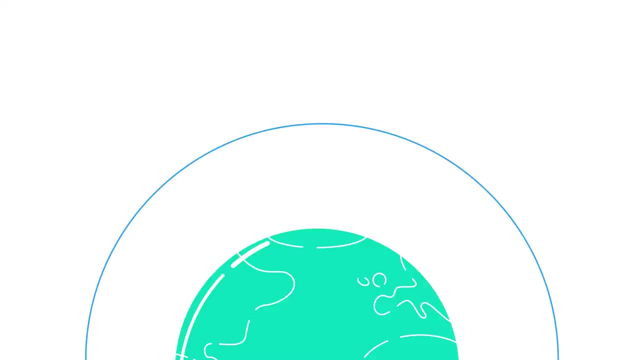 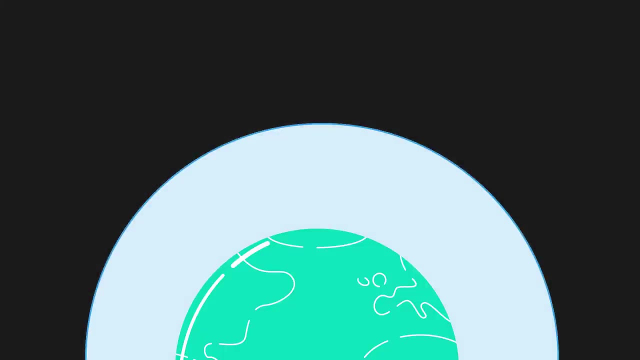 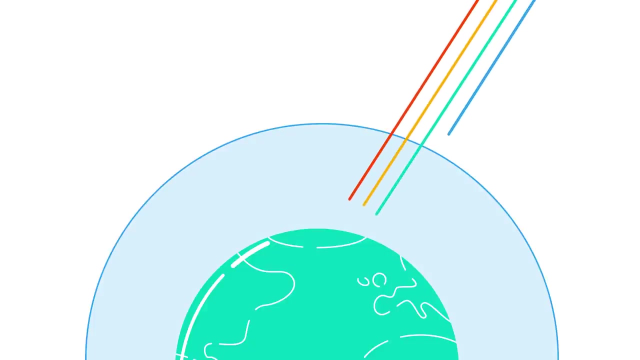 all fake. You wouldn't actually hear a thing As well as sound. we also have the atmosphere to thank for our sky being blue. Why do you think our sky is blue but space is black? Pause the video and have a think. The white light from our sun hits the molecules in our atmosphere.